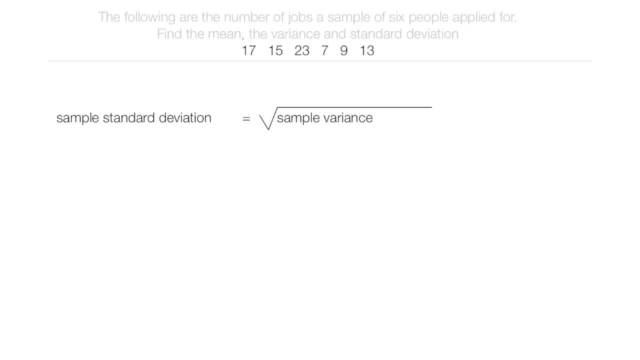 The sample standard deviation is equal to the square root of the sample variance, and these are the symbols I'm going to use. The first thing I'm going to calculate is the sample variance. The sample variance is this formula right here and we'll take the. 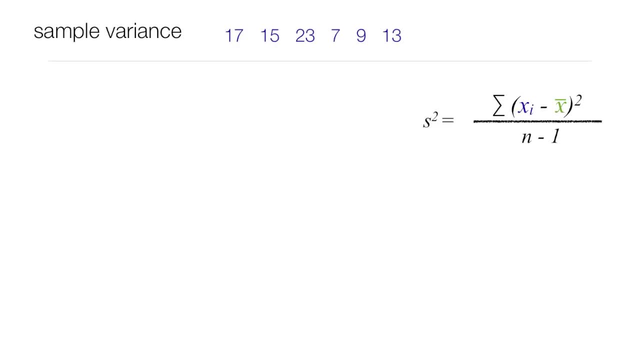 square root of that to get the standard deviation. The xi, that's the observations, The x-bar, that's the mean, and we'll go through the calculations of these. each one of these two and n is the sample size. I'm going to make a little table to. 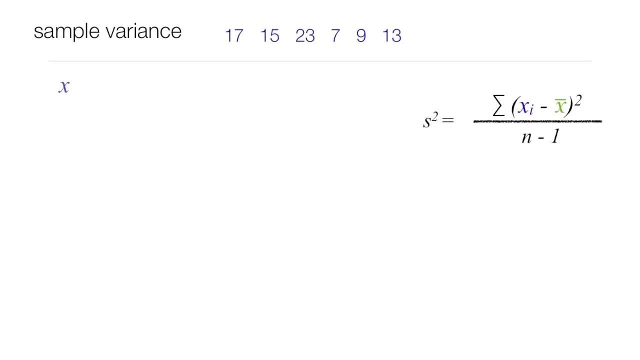 help me stay organized and I recommend that you do the same. I'm going to put in the x, which is my observation, and then we'll put a little line, horizontal line, and then I'm going to do an up and down vertical line as well. The next column is the mean x-bar. that's the. 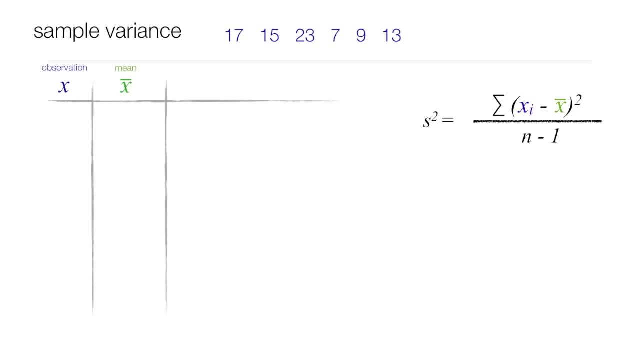 mean the sample, mean: Put a little vertical line as well. Now I'll just put in all the observations and that's the same as above and a line, and I'm going to put a couple more column headings in and you'll see, I'll tell you what those mean as 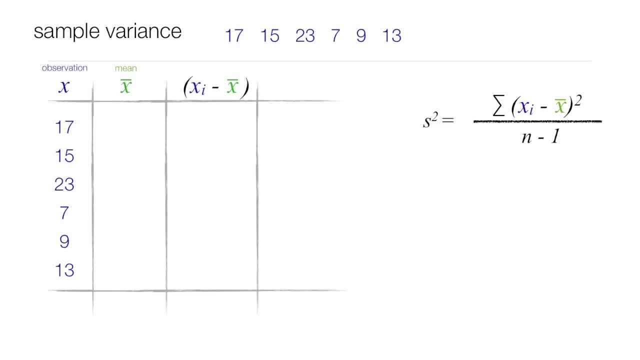 we fill them in but just go ahead and write them in now, And that's the observation minus the mean squared. So I need to calculate the mean, and that's equal to the sum of all my observations divided by the number of observations. 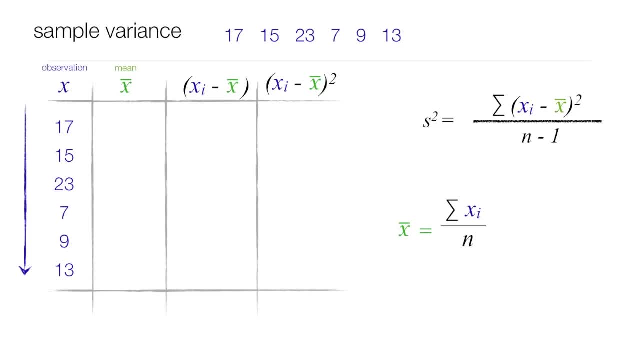 So if I add up all my observations, that column right there, that equals 84. Now I take that 84, and I put it right on top of that equation right there, and then that's my numerator divided by 6, and that equals my mean, which is 14 jobs. 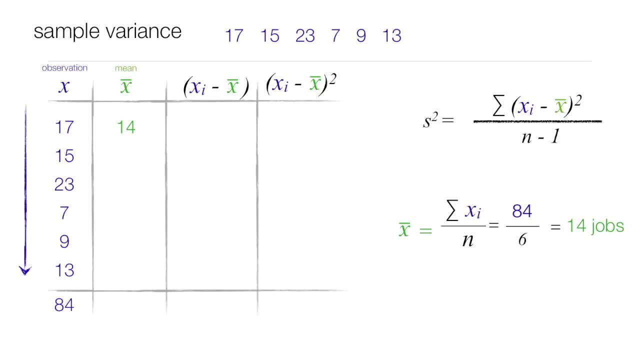 Now I take that 14 and put it right there in that column and the whole column is going to be filled with 14s. Now the next column over is the observation minus the mean, like 17 minus 14, and of course that is equal to 3.. 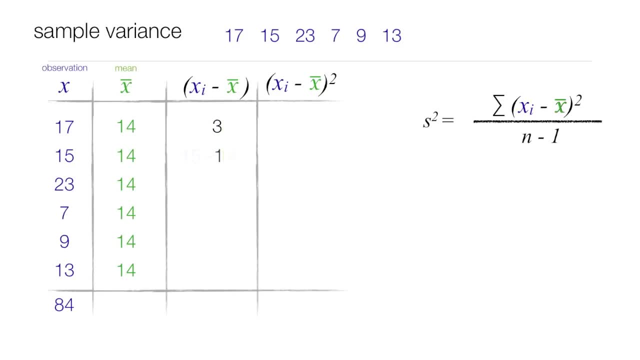 Then I have 15 minus 14.. That's equal to 1, 23 minus 14,, that's equal to 9, 7 minus 14,, that's a negative 7, 9 minus 14,, that's negative. 5, 13 minus 14,- that's negative 1..